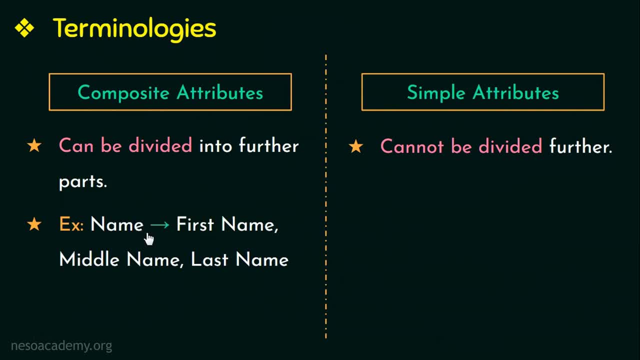 name. This attribute can be divided into further parts: first name, middle name and last name. An example of a simple attribute is weight. This attribute can be divided into further parts: first name, middle name and last name. An example of a simple attribute is weight This. 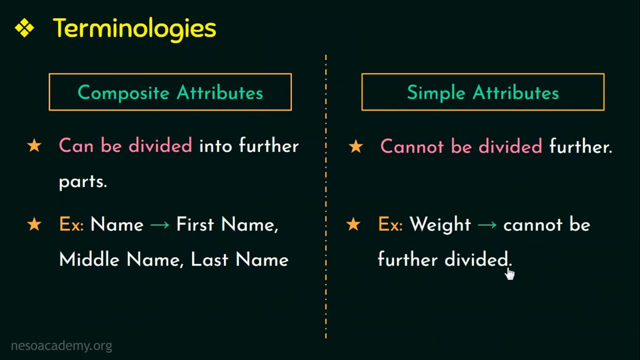 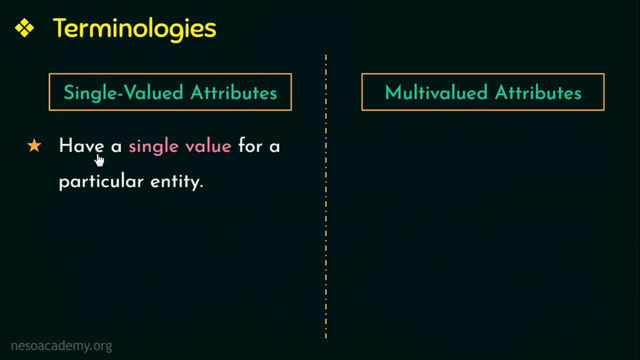 attribute cannot be further divided. Other examples could be salary, a person's age, etc. So this is about composite and simple attributes. Next we have the single valued attributes and multi-valued attributes. Single valued attributes are attributes that have a single value or just one value for a 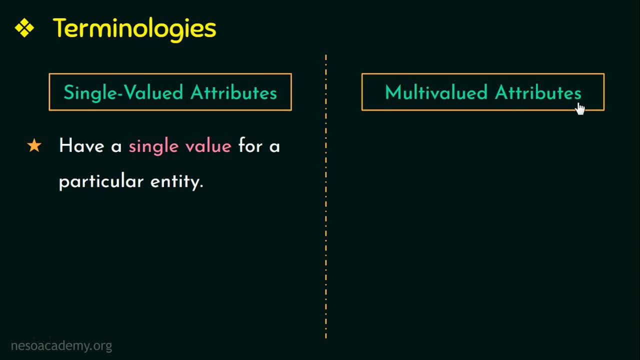 particular entity, whereas multi-valued attributes are attributes that can have a set of values for a particular entity. An example of a single valued attribute is value for a particular entity. An example of a single valued attribute is age. A particular person can have only a single. 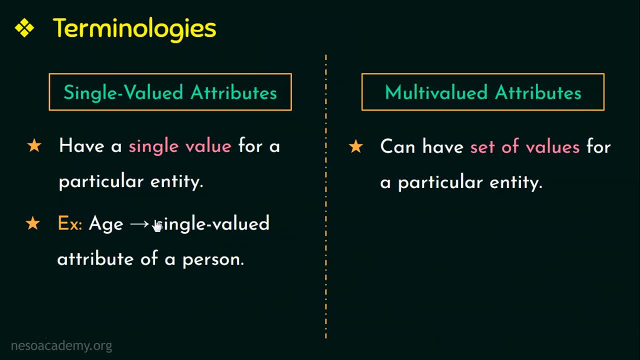 value for this particular attribute. So age is a single valued attribute of a person. The different types of multi-valued attributes are uses of. examples of multi-valued attributes are college degree, languages known, etc. A particular person can have more than one college degree and can also know more. 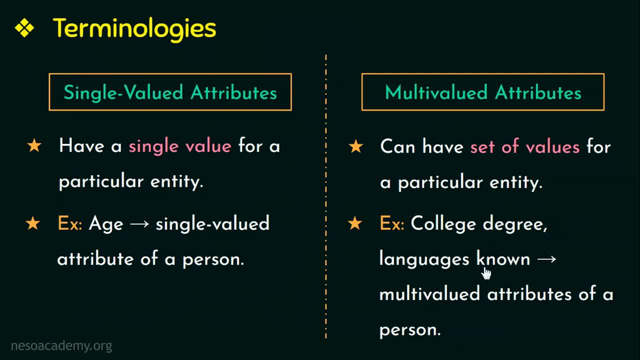 than one language. Since these attributes can have a set of values for a particular entity, it is called as the multi-valued attribute of a person. So these are about single-valued attributes and multi-valued attributes. Next let us see what derived attributes. 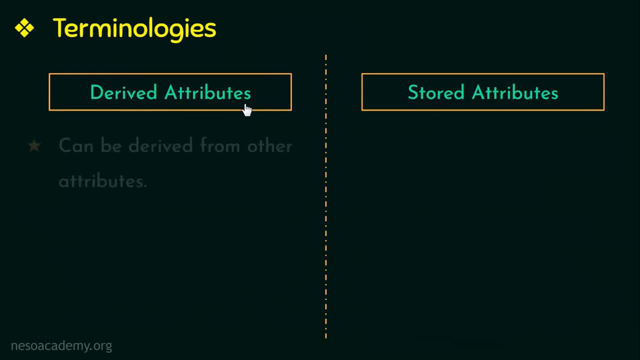 and stored attributes are Derived attributes are attributes that can be derived from other attributes, Whereas stored attributes are attributes from which the value of other attributes are derived. An example of a derived attribute is age. Since age can be derived from date of birth, this is called a derived attribute, Whereas date of birth or birth date of a person 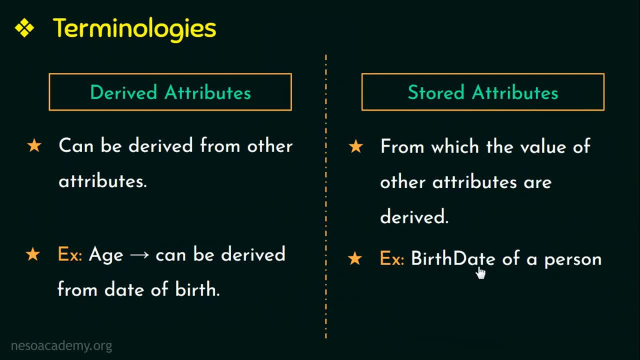 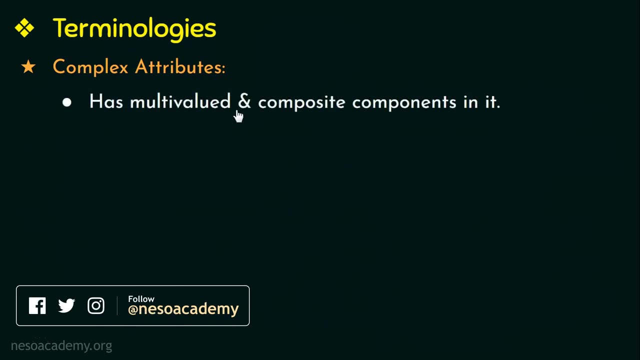 is a stored attribute because from this attribute we can derive age of a person. So this is a stored attribute from which the value of other attributes are derived. Next let us see what are complex attributes. A complex attribute has multi-valued and composite components in it. We have already seen earlier in this video. 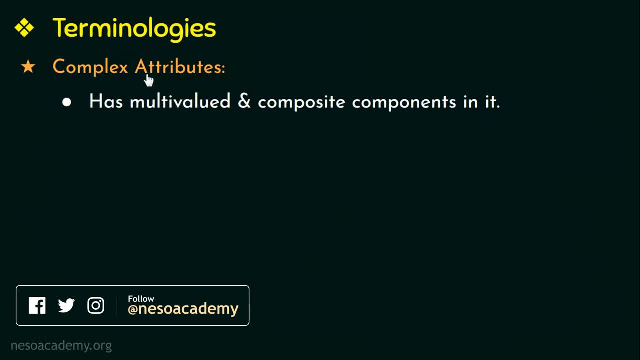 what multi-valued and composite attributes are. So a complex attribute has both multi-valued and composite components. Here, in the complex attribute, a multi-valued attribute is represented within curly brackets and composite attributes are represented within round brackets or parenthesis. This is an example of a complex attribute Here: college degrees. 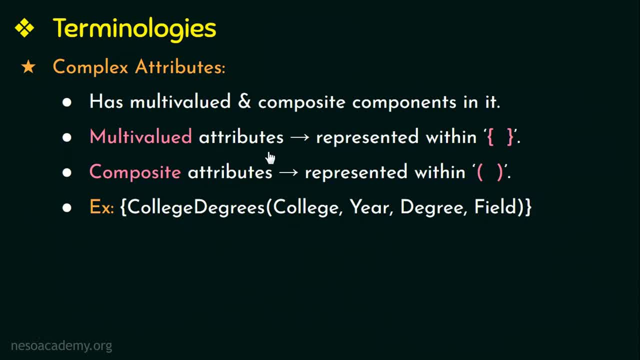 which is represented within curly brackets, is a multi-valued attribute, because one person can have more than one degree, And within the parenthesis is the composite attribute. So this is about complex attributes. Next, we are going to learn about null values: Null. 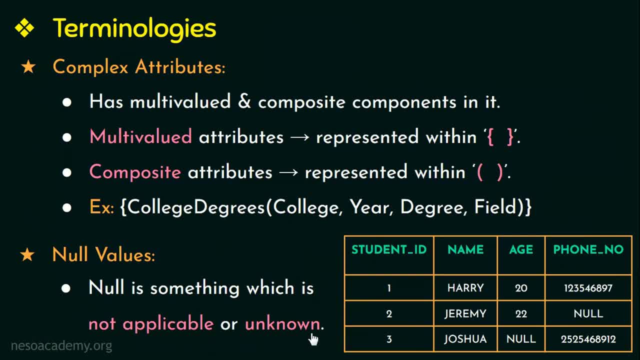 is something which is not applicable or unknown. So when does null value mean not applicable? In some cases, an entity might not have an applicable value for an attribute, Like, for example, if I have an attribute- college degree- this attribute applies only to persons with a college. 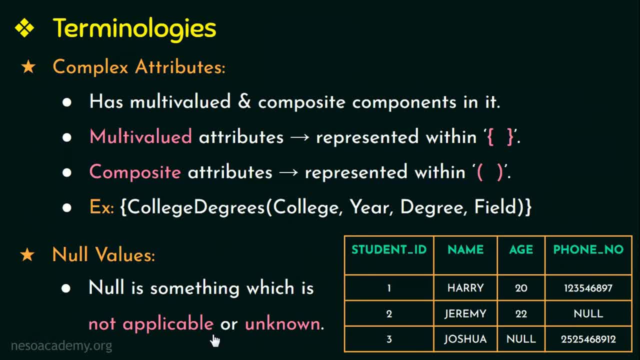 degree, Or if I have an attribute, say the landline number, this attribute again applies only to persons who has a landline. So a person who has no college degree will have null for the attribute college degree and a person who has no landline phone will have null for. 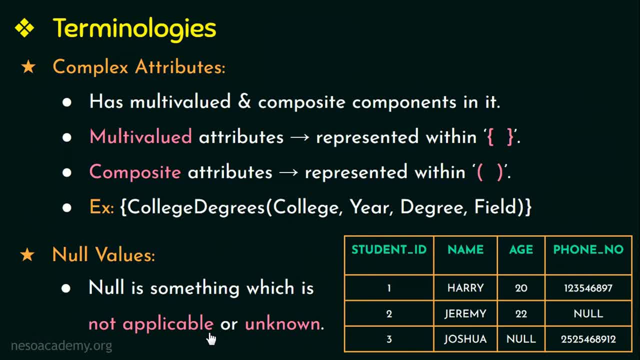 the attribute landline number. So in this particular case the meaning of null is not applicable. Null can also be used when we don't know the value of an attribute, Like for example, if we don't know the phone number of a particular entity here, say Jeremy, then that particular value of the attribute would 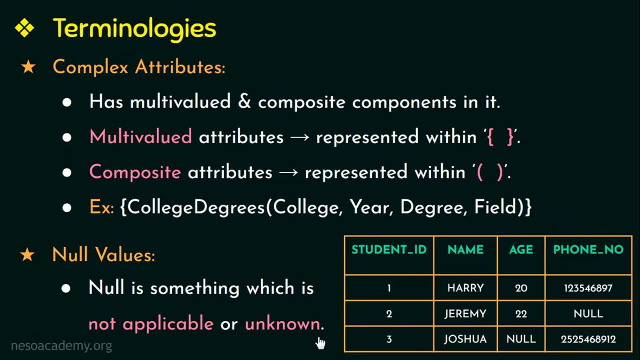 be null. So in this case the meaning of null is unknown. The unknown category of null can be further classified into two cases. The first case is when the value exists but it is missing, Like for example, the age of Joshua exists but it is missing. So that value would 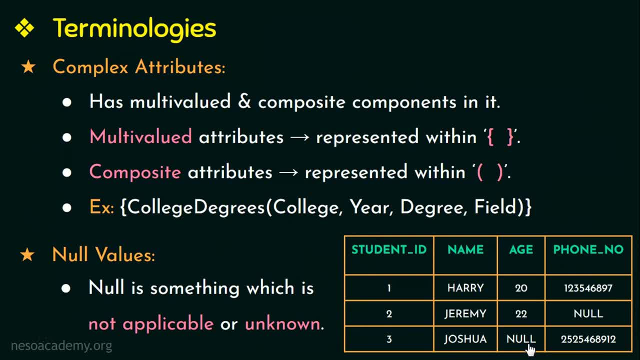 be null. The second case is when it is not known if the value exists or not, Like for example if we don't know whether the student Jeremy has a phone number or not. in that case, the value of the attribute phone number would be null. Hope you understood what null values. 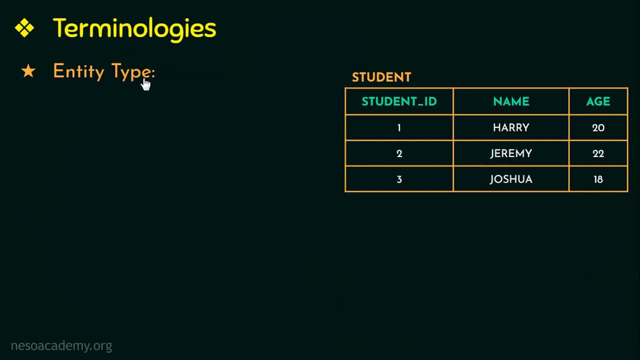 are. The next terminology that we are going to learn is entity type. What is entity type? It is a collection of entities that have the same attributes. Example of an entity type is: student. To record in this table is an entity. We have Harry, Jeremy and Joshua as the entities. 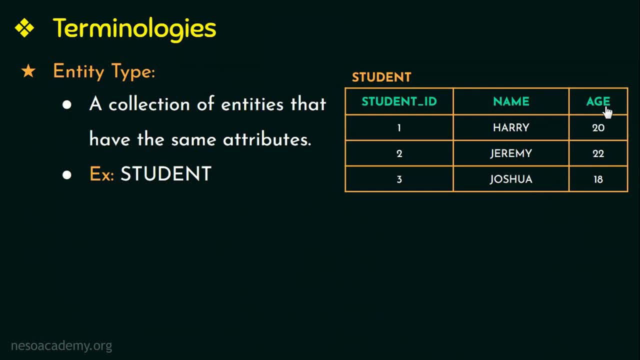 These entities share the same attribute, that is, age, and they belong to the entity type student. So an entity type is a collection of entities that have the same attributes. Now, what is an entity set? It is a collection of entities of a particular entity type. at 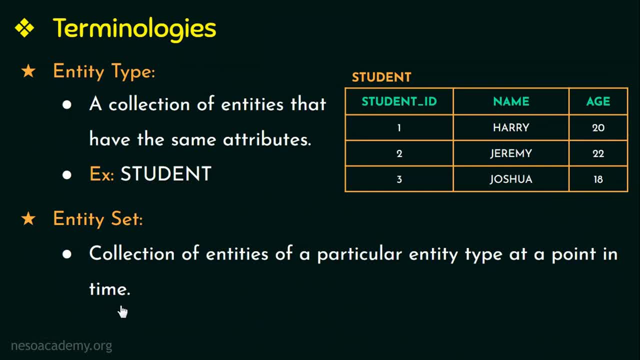 a point in time. If I say I need students whose age is between 19 and 23 years, I would say 19 and 23.. So at that particular point in time, all the students with age between 19 and 23 is an entity set. 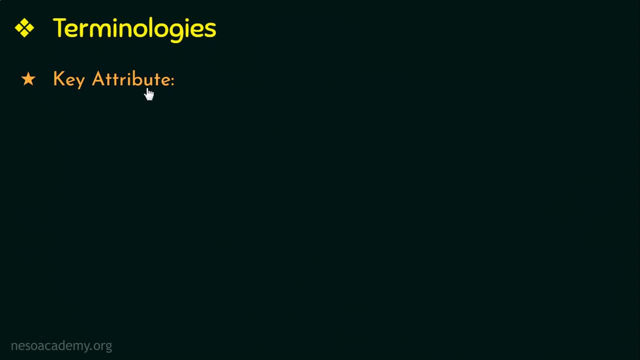 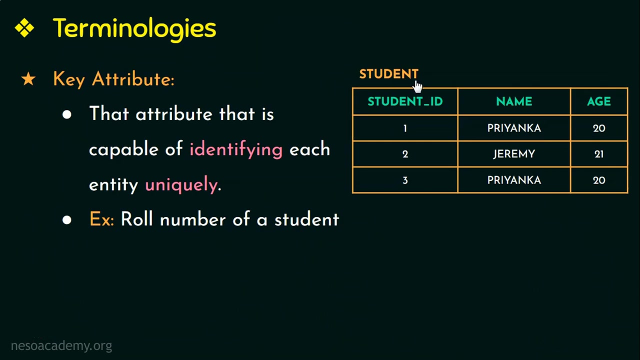 Next, let us see what a key attribute is. A key attribute of a particular entity type is that attribute that is capable of identifying each entity uniquely. For example, role number of a student. Now in this table, with entity type, student, I have two students with the same name and 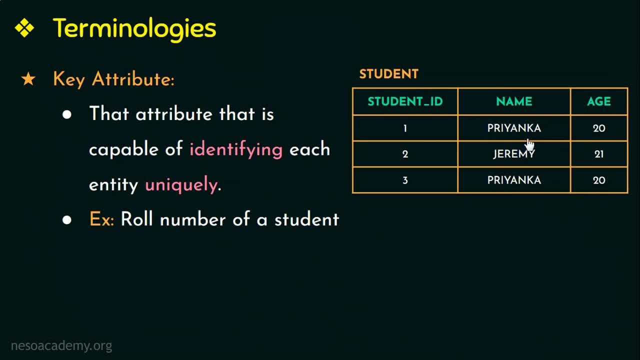 also the same age. If I have to identify this particular student uniquely, I can identify her by her student ID or role number, because no two students can share the same role number in a particular class. So the attribute role number or student ID is a key attribute to identify a student uniquely. 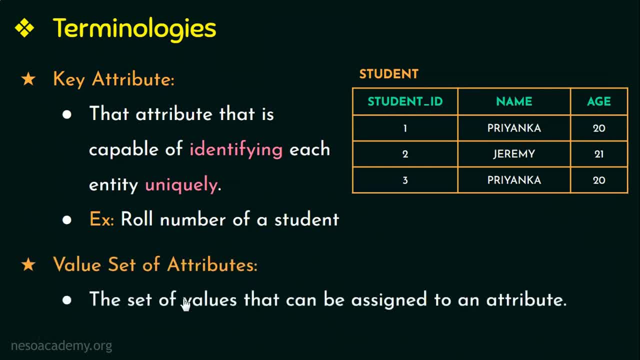 Next, what is value set of attributes? Value set of attributes is a set of values that can be assigned to a particular attribute. For example, if the range allowed for the age of an employee is between 22 and 60,, then we can specify the 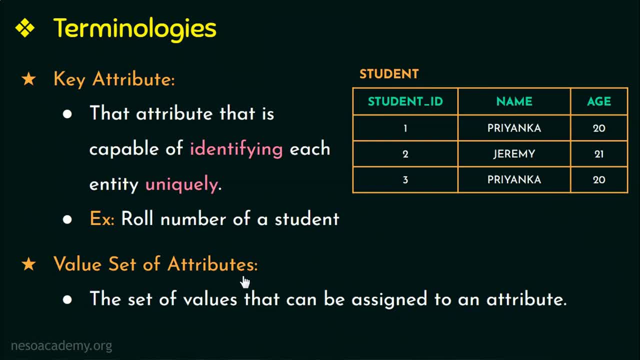 value set of the age attribute of an employee as a set of integer numbers between 22 and 60. So that is called as a value set. So these are the few important terminologies that we need to know in relation to the ER model. 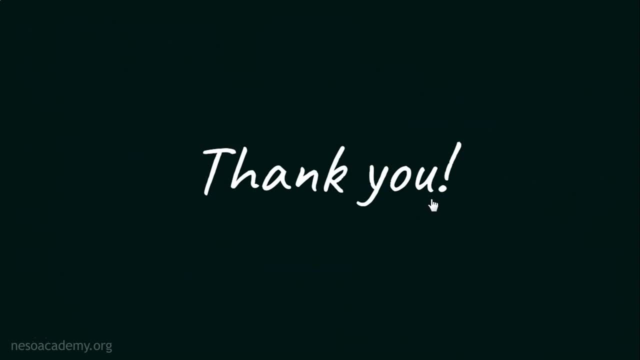 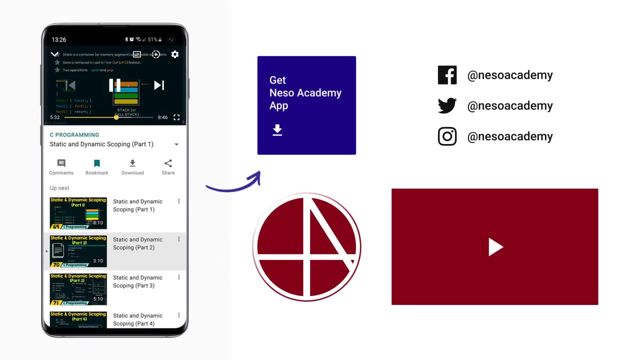 With this we come to the end of this video. Hope you have understood the definition of each of these terminologies, Thank you. Thank you very much for watching and we will see you in the next video.